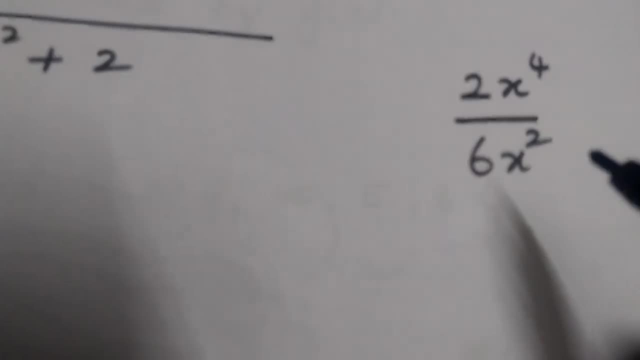 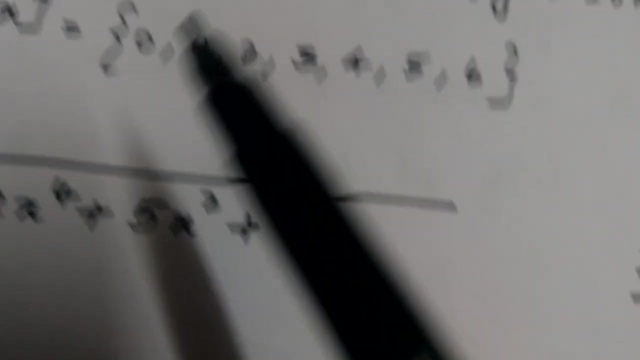 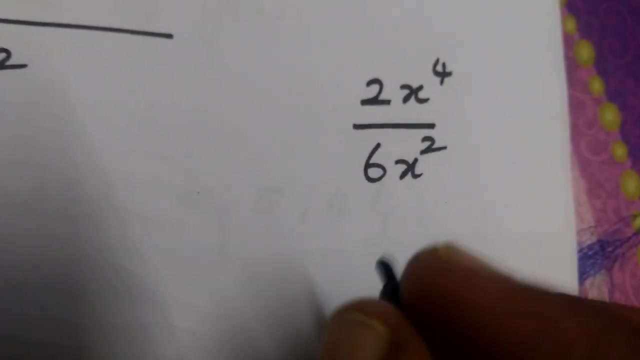 what am I supposed to do? How to solve? How to solve when you have fractions? So what do you do? First, you go to the modulo number. What is the modulo number given in the problem 7.. So, first, what do you do? I will. 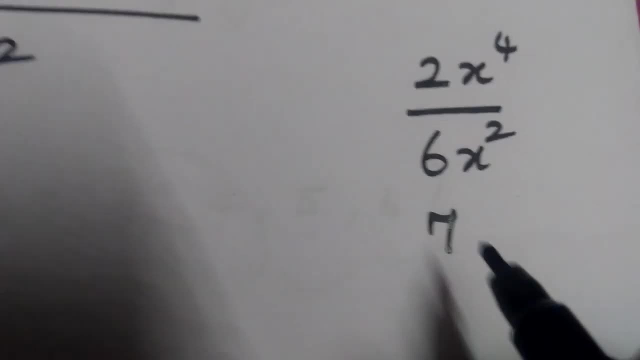 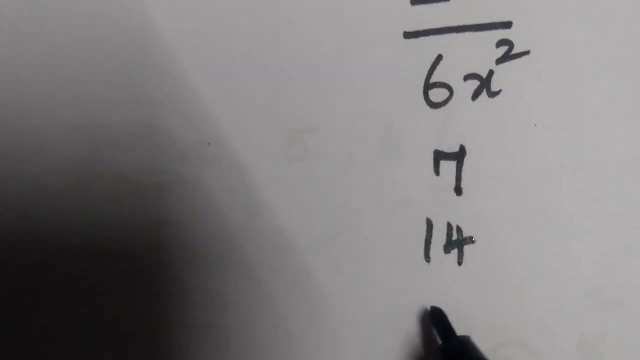 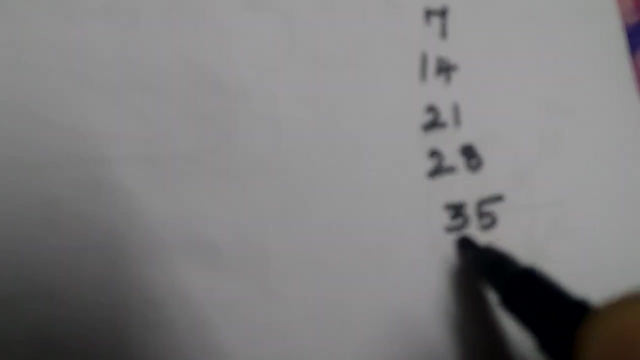 write 7.. So first I will write 7.. 7 times table 7.. What is the next number 14.? What is the next number 21.. What is the next number? 28,, 35 and so on. You just keep going Right Now. what will I do? How to solve in this category? 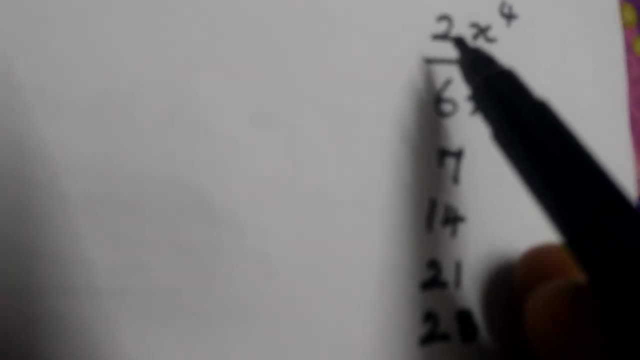 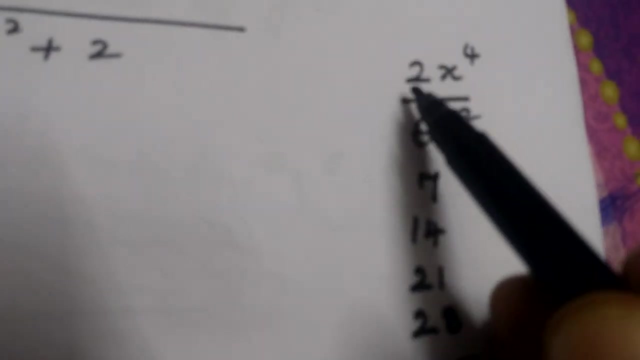 I need to know: from where did this 2 come from? This 2 is the reminder. Okay, So now, what will I do? Now, you got to see what number is here. The number 2 is here. So what will I do? I will. 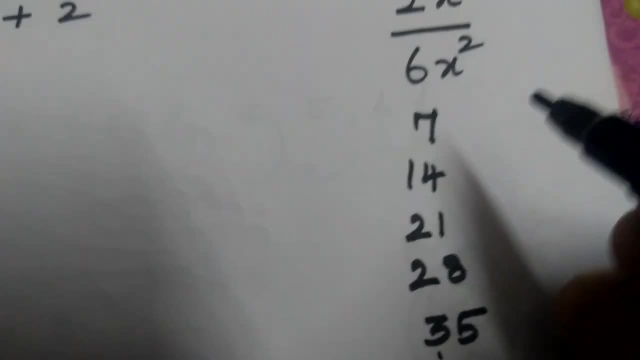 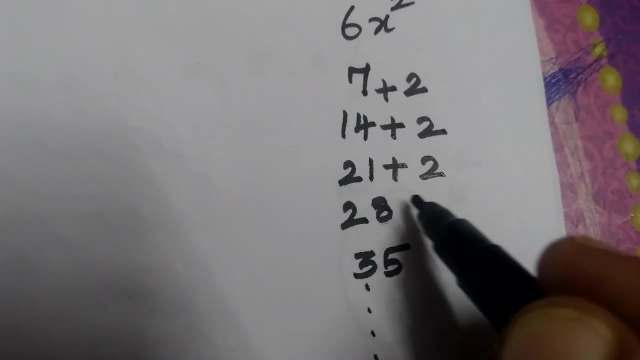 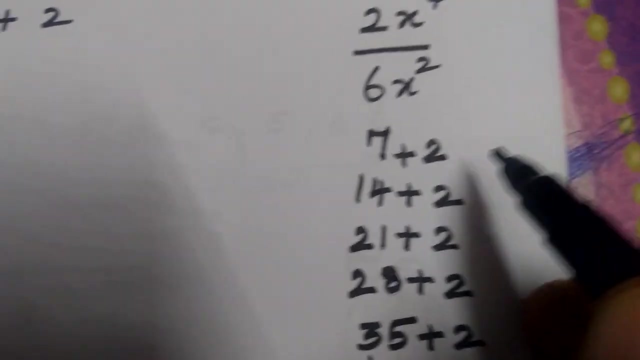 add up this 2 to every of the number, So now 7 plus 2.. 21 plus 2.. 28 plus 2.. 35 plus 2.. Etc. Now what are my answers? Can you tell me the? 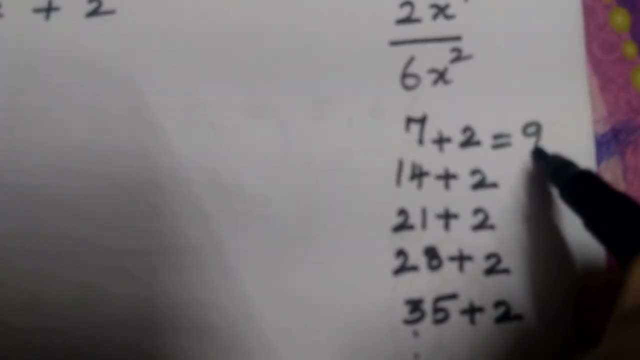 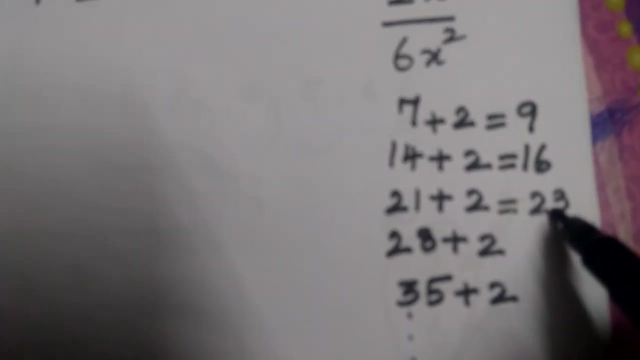 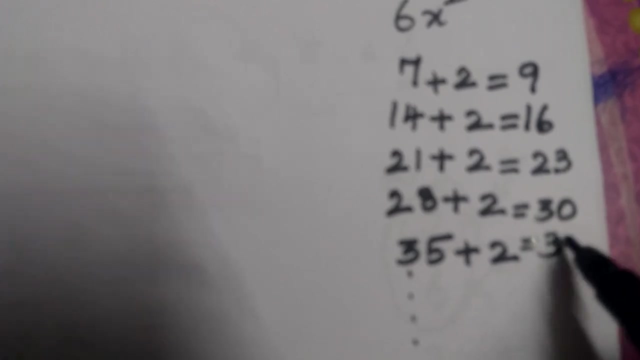 answers: 7 plus 2 will give you 9.. 14 plus 2 will give you 16.. 21 plus 2 will give you 23.. 28 plus 2 will give you 30.. 35 plus 2 will give you 37, and so on. Now, what is the next number? 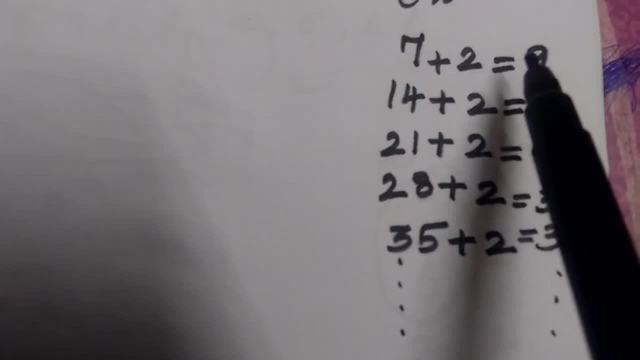 Okay. So what is the next number? 8 plus 2.. 28 plus 2.. 35 plus 2. Etc. Now, what is the next number? What will I do? I will choose a number from this particular set so that it is perfectly divisible. 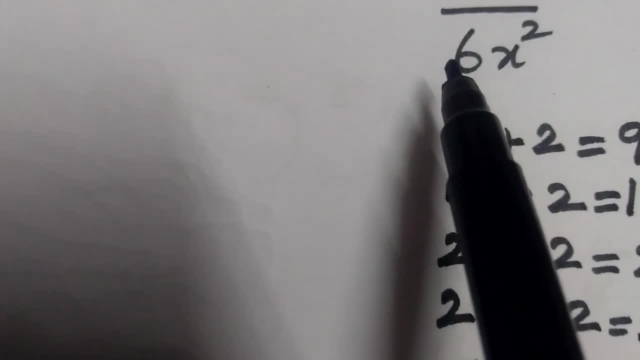 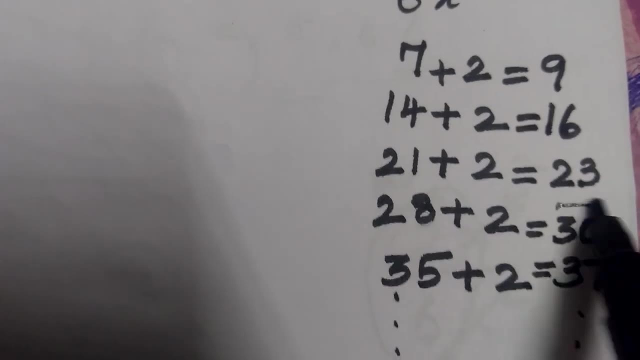 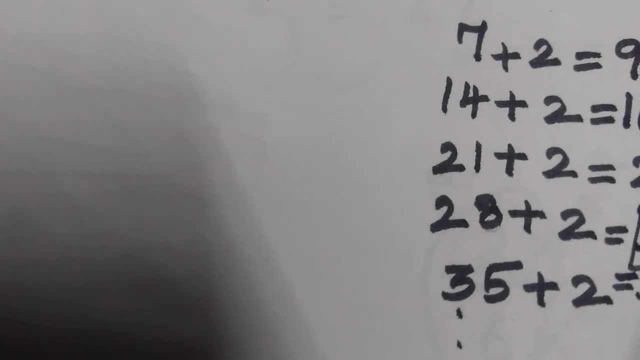 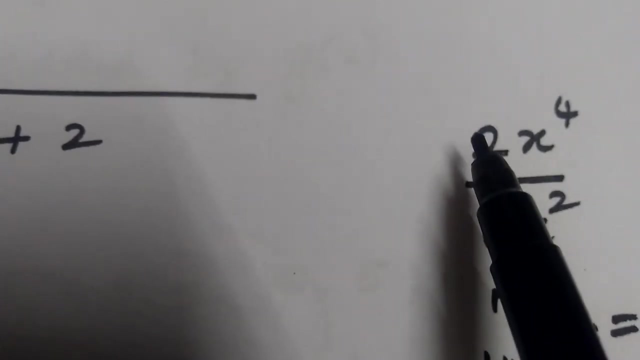 by the number 6 which is in the denominator. So what number it is? Except the number 30, you will not have any other number divisible by 6.. So 30 is the perfect number which is divisible by 6.. So I will replace this 2 by 30.. Very simple, I will replace this 2 by 30.. So now it has become. 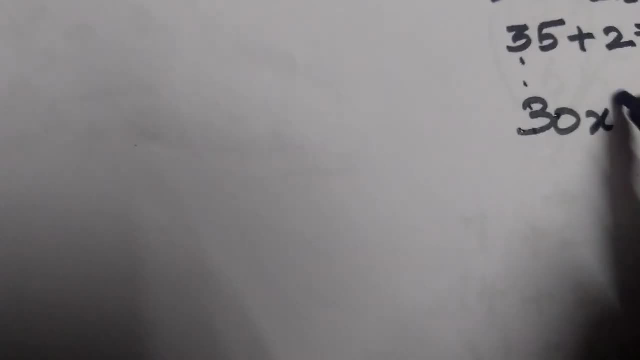 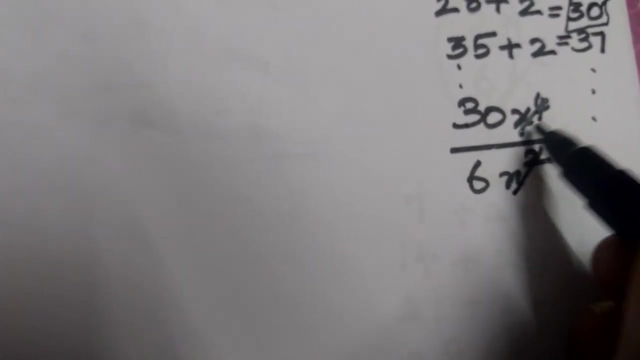 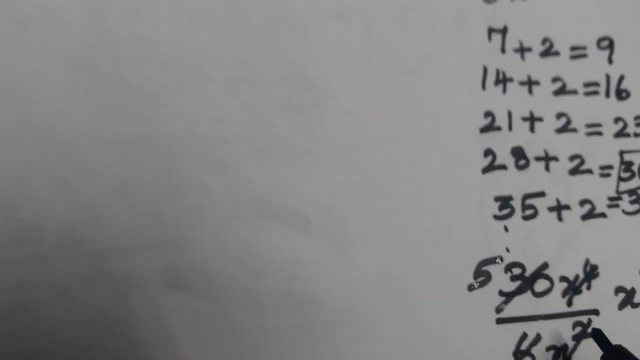 30 x power 4 over 6 x square. So if that is the case, x square and x power 4 will get cancelled. I will be getting x square and 6 will get cancelled 5 times. So what is the number I am arriving at? 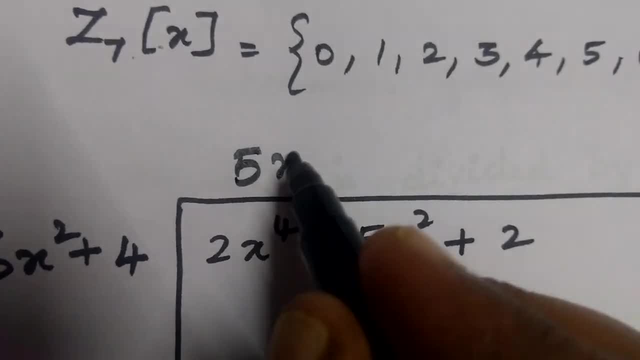 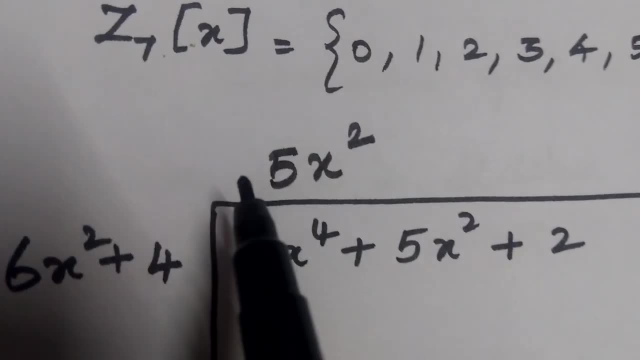 5 x square. So here in the quotient place I will be writing 5 x square. Now take 5 x square and multiply. If I am going to multiply, I will be getting 5 into 6, will give you 30 x power 4. But 30 is not. 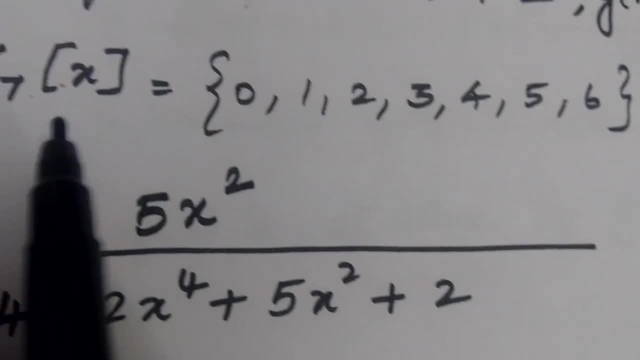 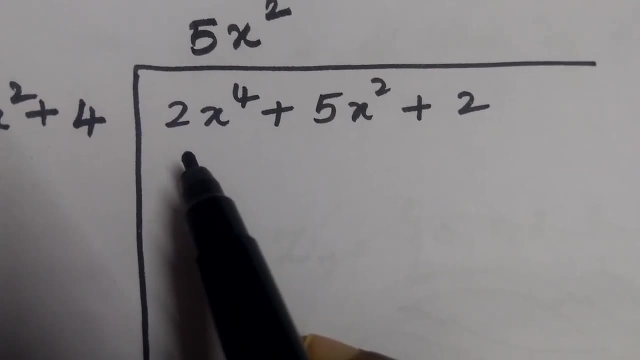 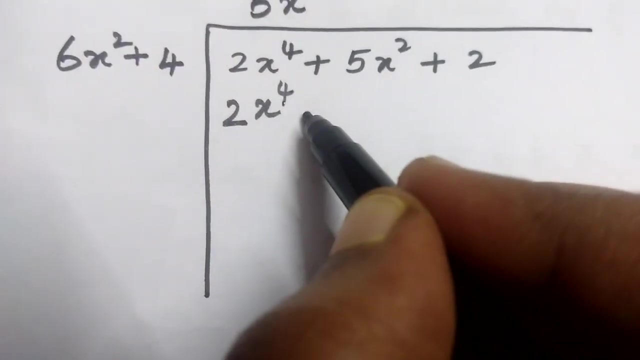 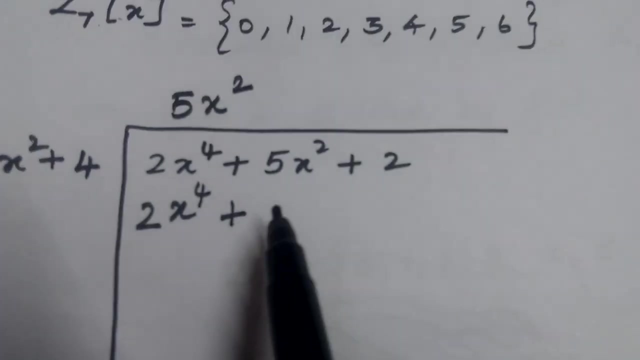 allowed here. Since it is modulo 7, I got to divide that by 7.. So 30 when I divide by 7, which is 28, and the remainder is 2. So you write the remainder 2 x power, 4. Plus 5 into 4.. 5 into 4 will give you 20.. Is 20 allowed here? 20 is also not allowed. Divide that. 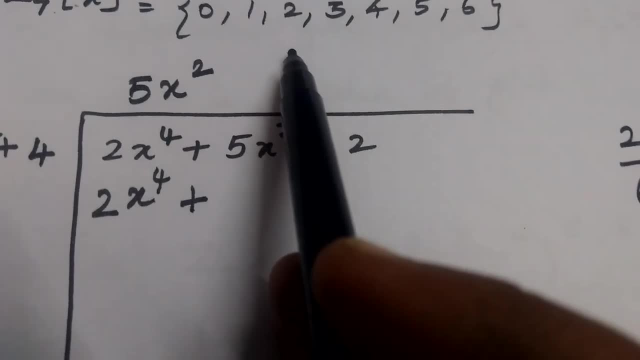 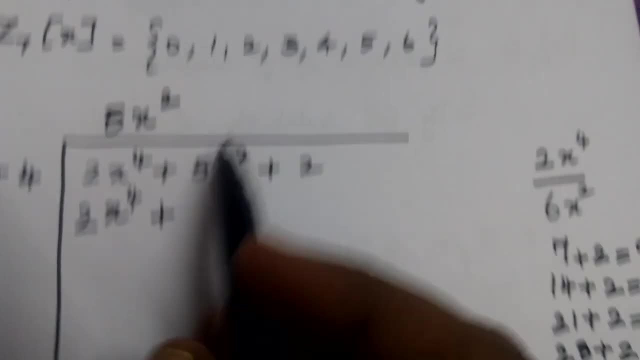 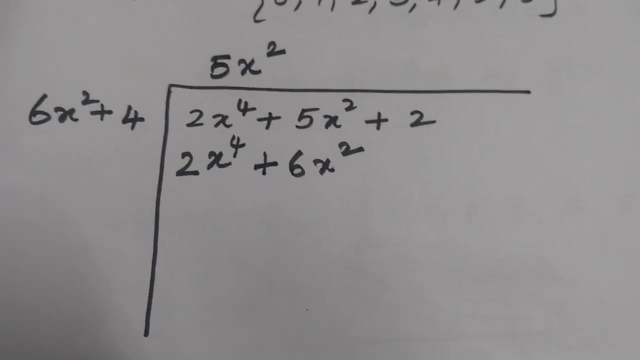 by 7.. What is the closer number to 20?? I will be getting 14.. So what is the remainder? Reminder is 6.. So I will be writing 6 x square. Are you able to follow? So first I will see, First I will generally. 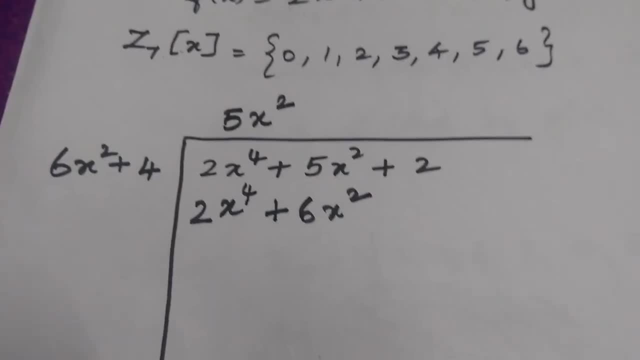 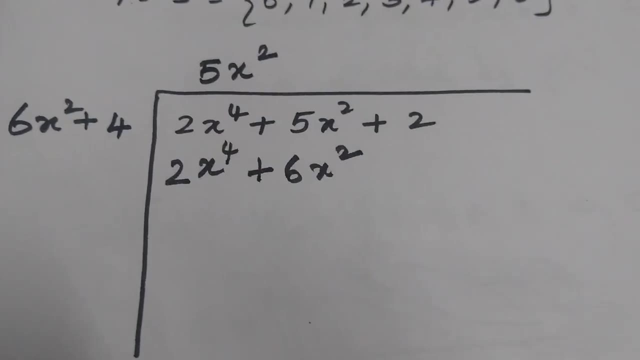 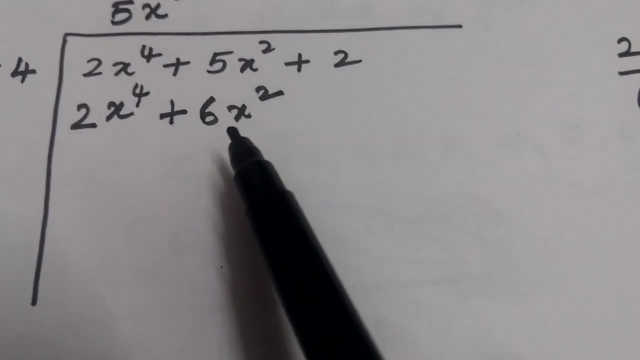 multiply it. Since the number is not allowed in the modulo set, I will write the divide by that particular modulo number and write the divide, sorry, the remainder. So 4 into 5 into 4 will give you 20, and 20 is divided by 7.. So 14.. So remainder is 6.. Now what do you? 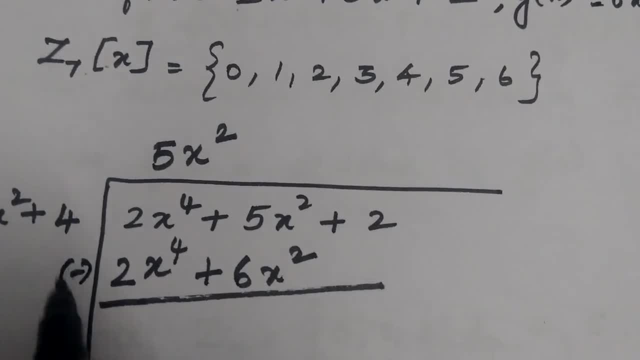 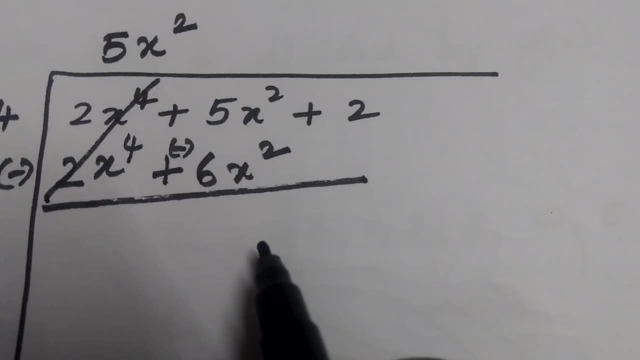 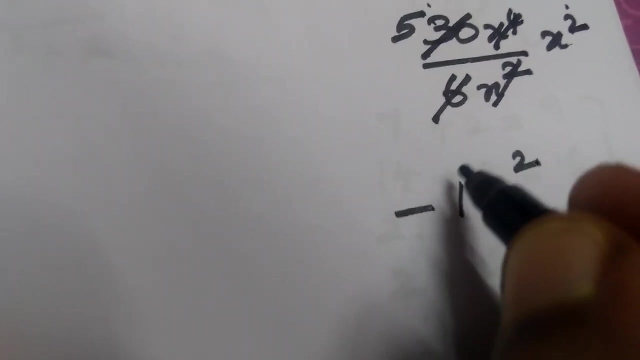 do Change the sign, Cancel this out. So what are you getting here? I am getting minus 1 x square. So what is the closer number to 20?? I will be getting minus 1 x square. So again there is a problem. So here, since minus 1 x square, you are having negative numbers are. 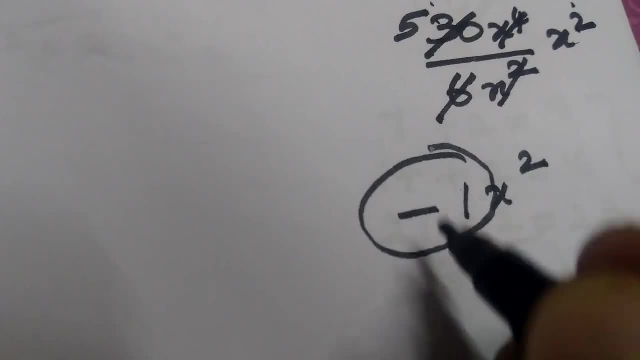 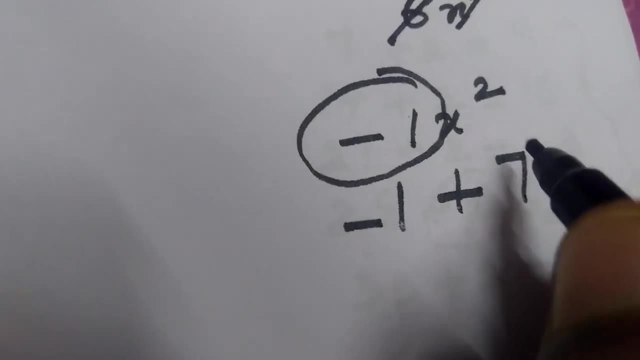 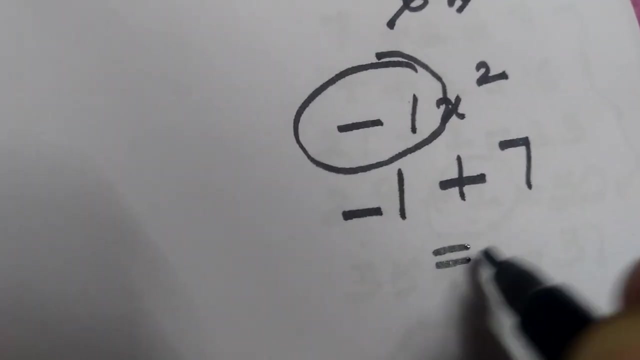 not allowed. So what will I do? I will subtract this from the modulo number. What is the modulo number? I am having 7.. So put 7.. So use the modulo number to convert a negative number to a positive number. So minus 1 plus 7 will give you 6.. So that 6 will be carried out here. 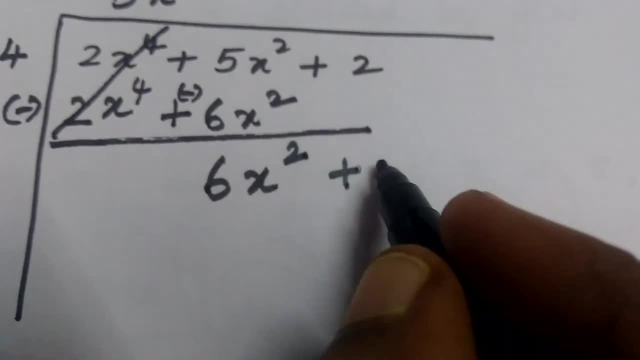 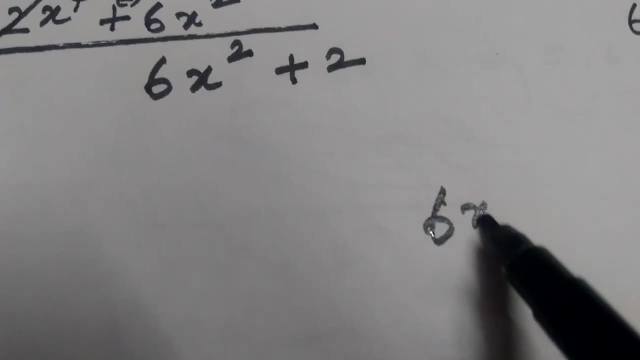 So 6 x square. Bring down this. 2. Now take the 6 x square and divide it by 6 x square. So if I am going to divide 6 x square over 6 x square, I will be getting cancelling out both. I will be getting. 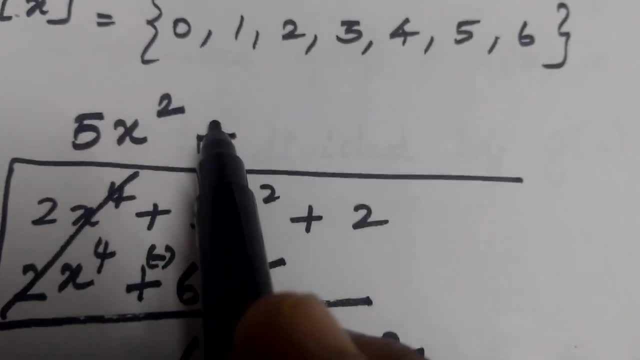 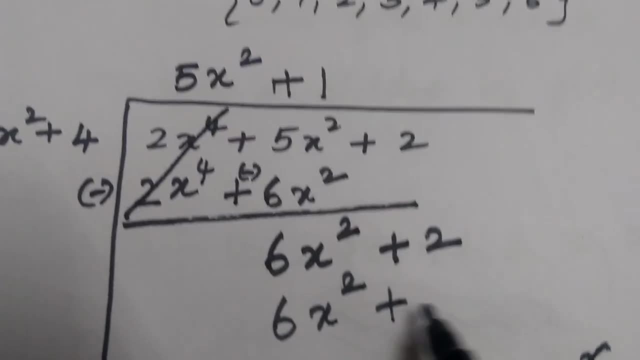 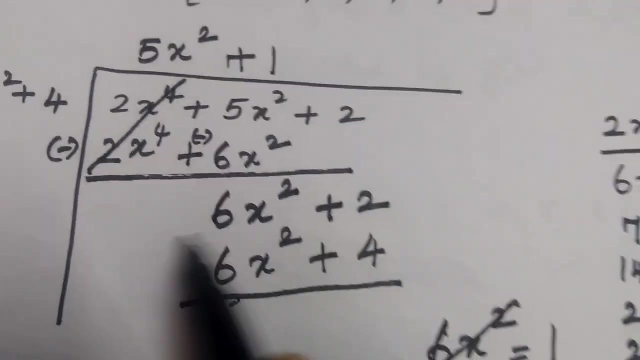 1.. So write that 1 in my quotient. Now take this 1 and multiply by this number, So you are getting 6 x square plus 4.. 6 is allowed in the set, So I am just keeping it. Changing the sign, Cancelling out, Changing the. 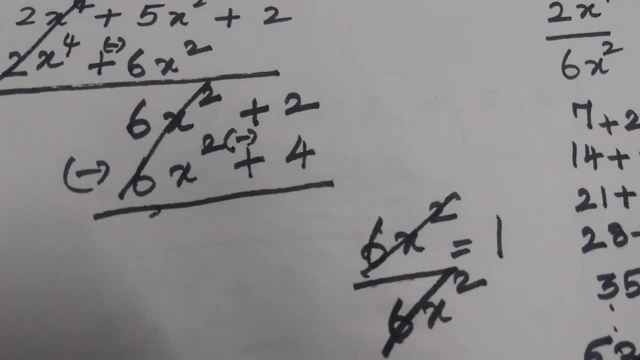 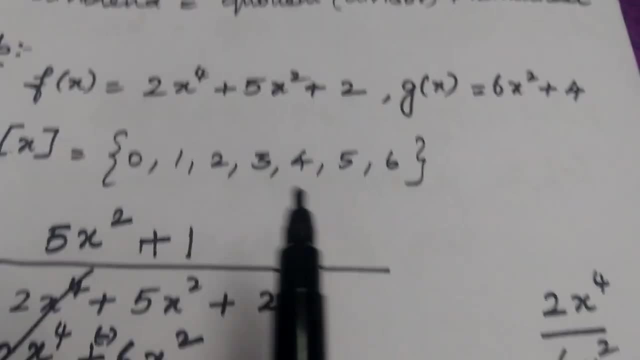 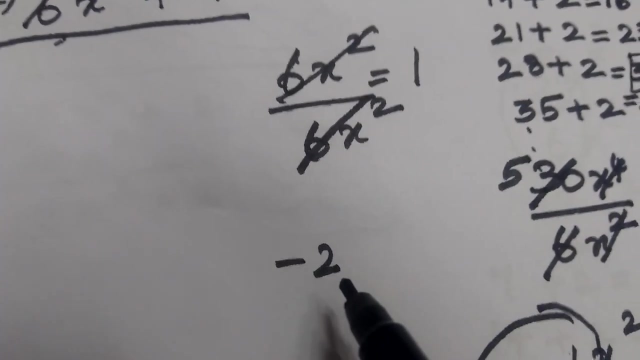 sign. What is my answer? A negative number, Minus 2 I am getting. So is minus 2 allowed? Definitely not. There is no negative number here. So what will I do? Since my number, since my answer reminder, is becoming minus 2, I have to convert it into a positive number. So how will? 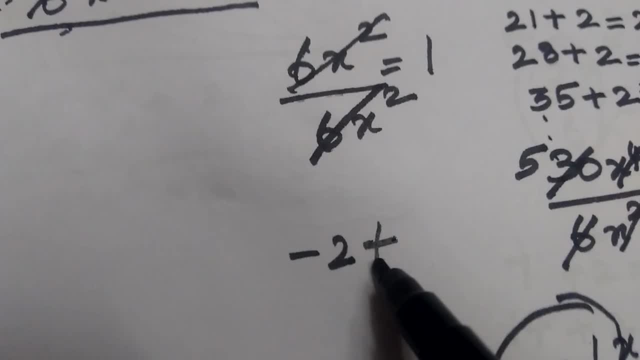 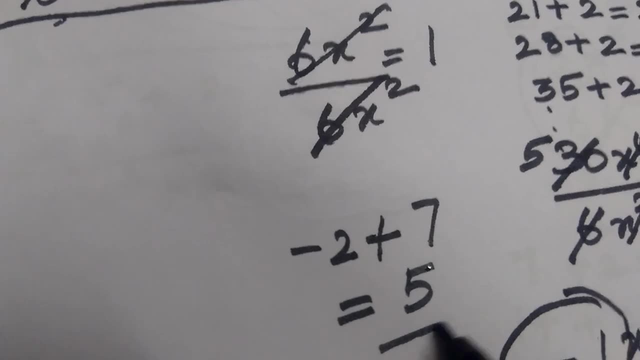 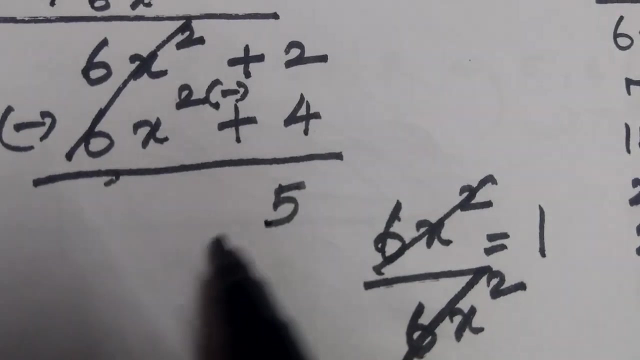 I convert it into a positive number Minus 2 plus the modulo number Adding it. So if this will be, my answer will be 5.. So my negative number is getting transformed into a positive answer, So my answer is 5.. This is the reminder, This is the 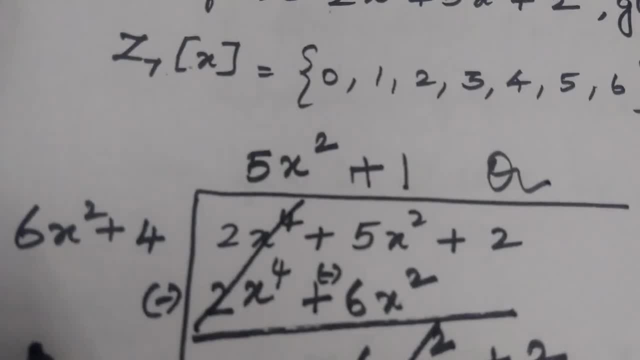 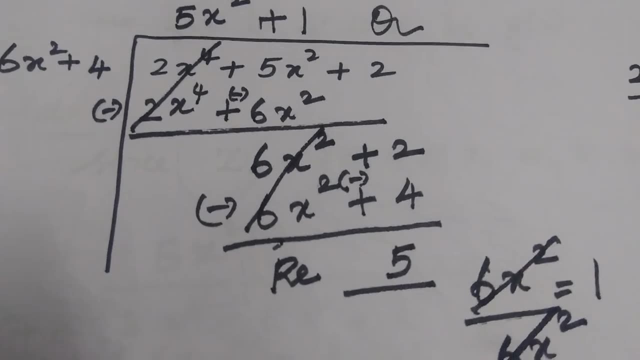 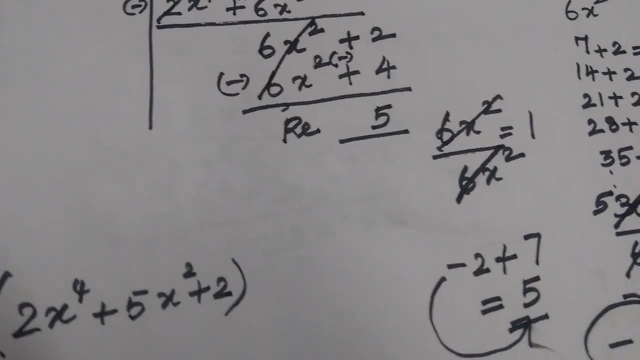 quotient And this is my divisor and this is my dividend. So therefore, by division algorithm, I can write it as 2 x power, 5. 4 plus 5 x square plus 2.. Ok, No, need bracket, I just accidentally put it up. No issues, If you use it also, no issues. 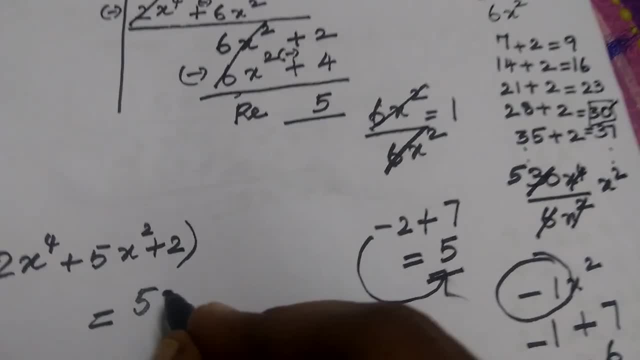 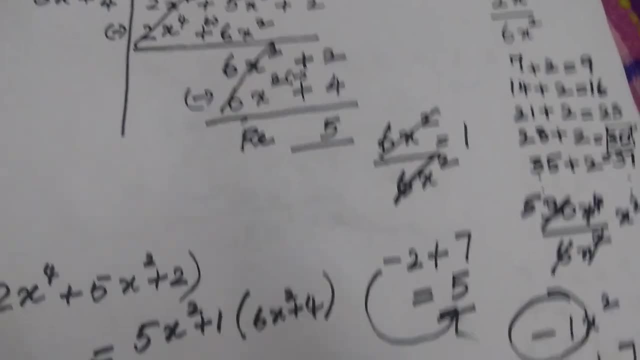 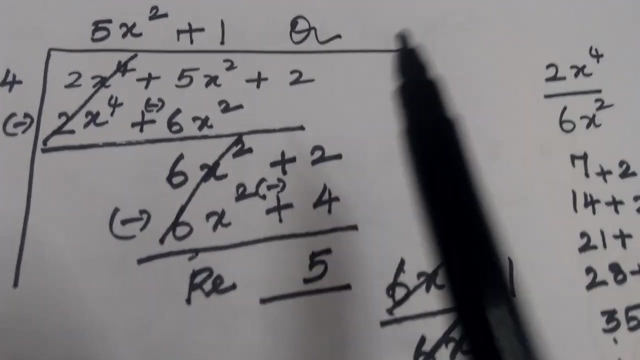 So it is going to be. the quotient is 5 x square plus 1 into the divisor, 6 x square plus 4 plus 5.. So this is my answer for the division algorithm. I hope all the things are clear, So always remember. 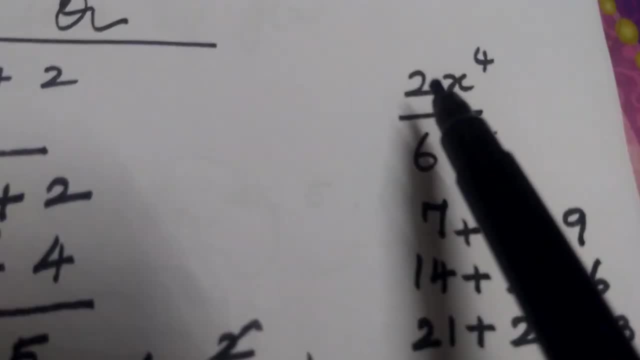 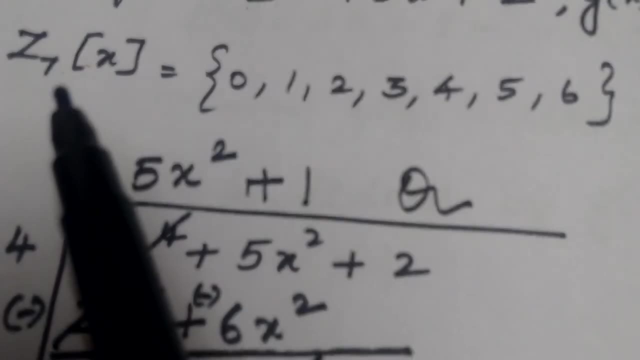 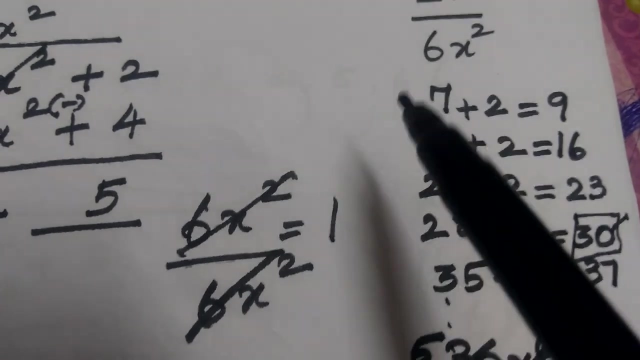 whenever you have a lesser number on my numerator, what you do? take the modulo number. whatever it may be The problem in this problem, the modulo number was 7.. Suppose, if the modulo number is 5, write 5 times table. So I think this will be easier step for you: Write the 5 times table and add up that particular. 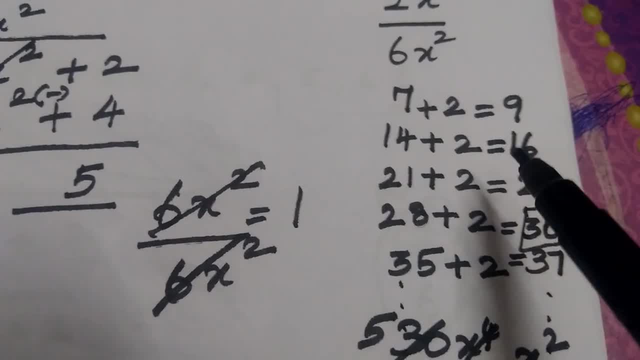 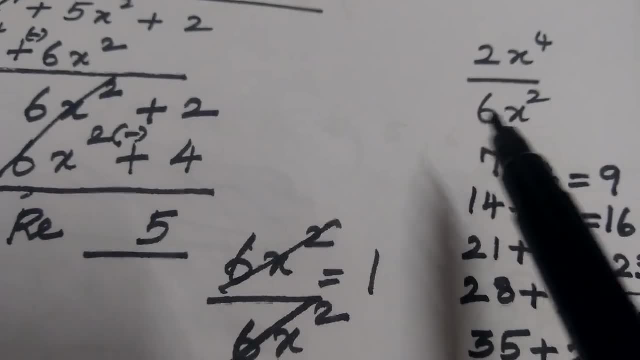 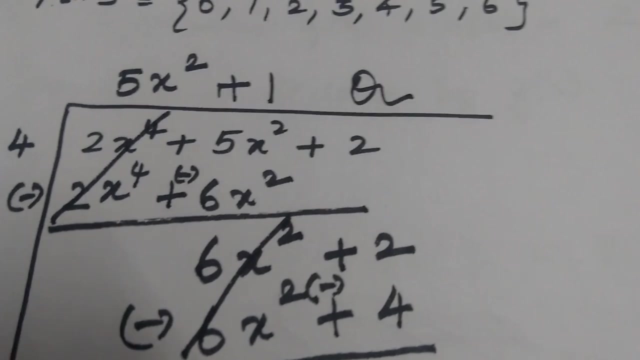 2 to whatever number is there in the numerator and get the answer and see which answer exactly gets divided by the denominator. So choose that number, divide it and then get the particular answer. That answer will be there, Thank you.